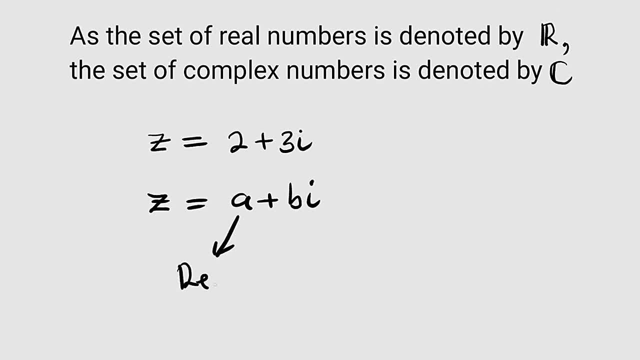 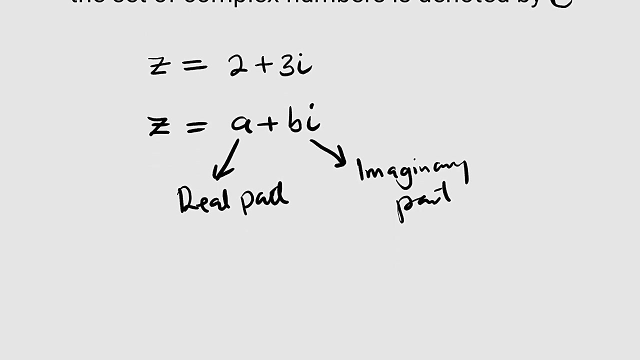 a right here is the real part, while b? i right here- is the imaginary part. but some people might ask: we have seen that b is a real number. why should we call b? i the real number and why should we call b the imaginary number, the whole of b? i to be the imaginary part? b is just a multiple of i because i is an imaginary. 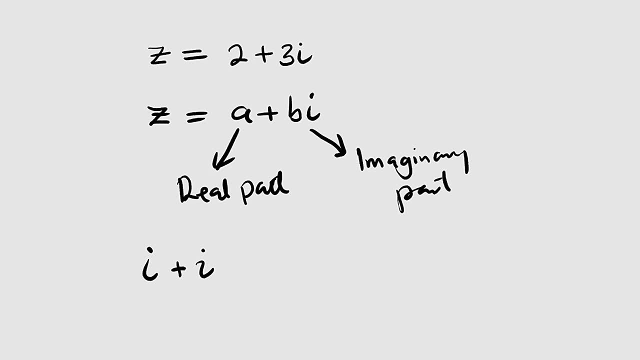 number. if you add it to another i. both of them are all imaginary numbers. together you have two of them to i. therefore, two here, which is a real number, is just a multiple of i, which determines the quantity of i in that part. but if you want to be specific about these real numbers, a 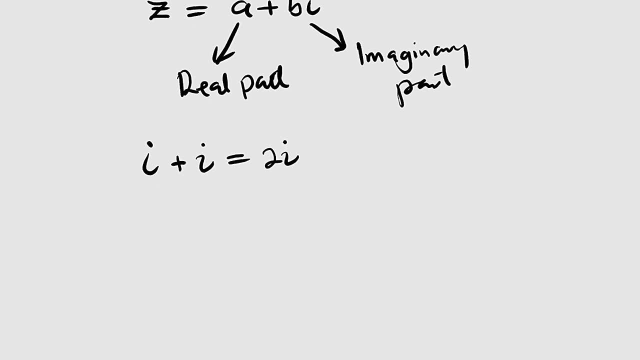 and b. this is how you can identify them. the real part, re, of z is equal to a. that is the real part of the complex number. z is equal to a and the imaginary part of this z is just b, that is the multiple of our imaginary number. here is b. we are talking about the imaginary part of z. it's only the. 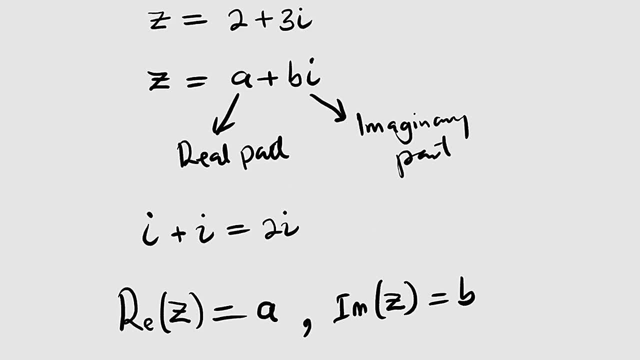 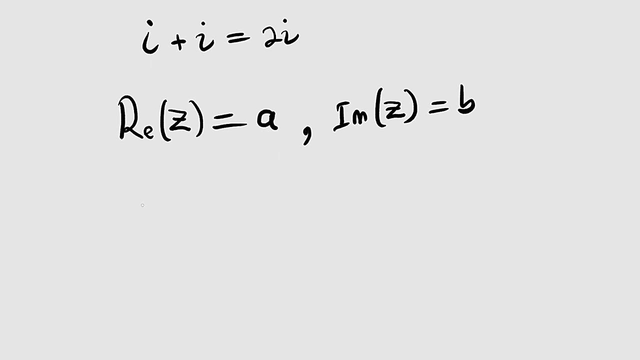 coefficient of that i. but the real part is always the first time here. but the one thousand dollar question here is that is a real number, a complex number or is an imaginary number? considered as a complex number? yes, because, um, if z is equal to a plus b, i, what if a is equal to 0? we know that 0 is. 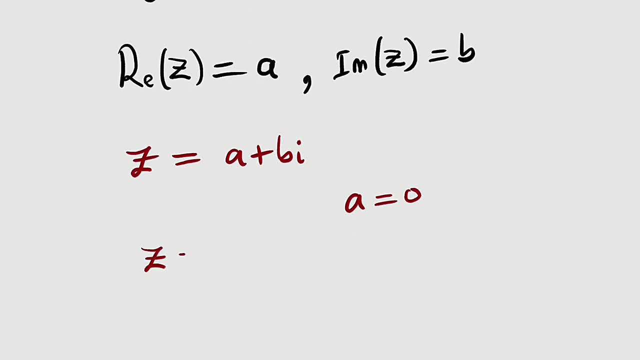 a real number, then the real part is always the first time here, but the one thousand dollar question. therefore, we have z equal to 0 plus b? i. so you can see this is just an imaginary number, b? i, which is also considered as a complex number because the real part is equal to 0.. so what if b?